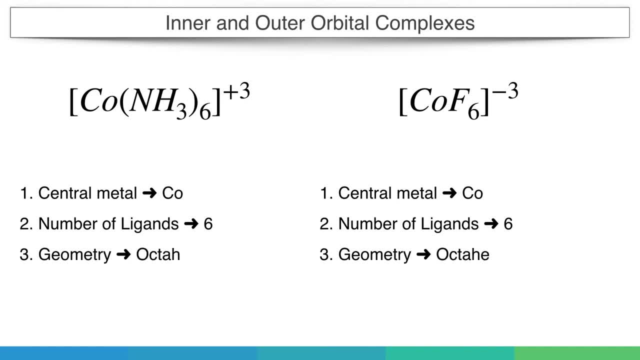 properties of these two were analyzed, it was found that the hexamine cobalt 3 is dimagnetic, while hexafluorocobalt 3 is paramagnetic in nature. As magnetic behavior of complexes are directly linked to unpaired electrons, it is clear that both the complexes 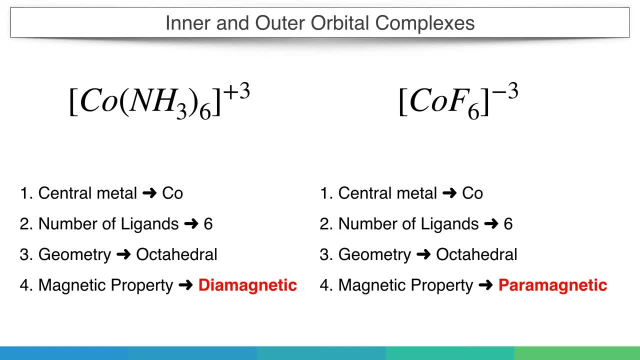 are having different numbers of unpaired electrons. That means they are not having similar type of bonding, Even if the central metal is same and number of ligands are also same. This strange behavior can only be explained with the concept of inner and outer orbital complexes. 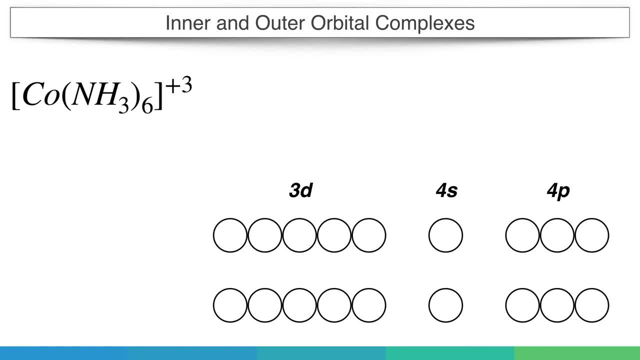 Let's try to explain the bonding. in first complex We can calculate the charge on cobalt from the charge on molecule and charge on each ligand. So in this case cobalt is in plus 3 oxidation state. As atomic number of cobalt is 27,. its electronic 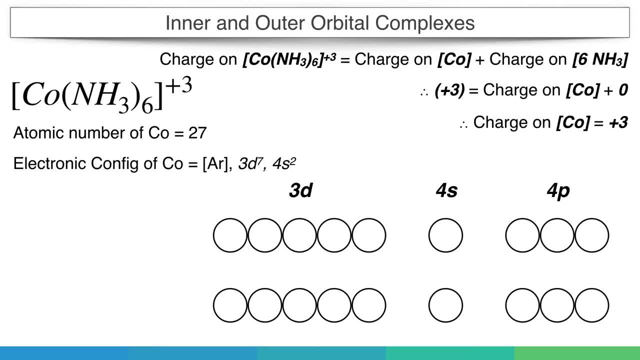 configuration will be Argon 3d7, 4s2.. 3 electrons will be lost as cobalt is in plus 3 oxidation state, So the electrons can be filled in orbitals of 3.. In this case cobalt is not in plus 3, but it is in plus 4 oxidation state. 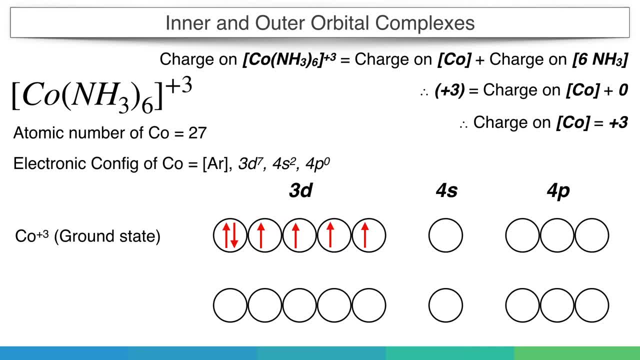 we can discuss about the cobalt in real time. Now we can see that the 2 electrons of cobalt are empty in the first place. However, since there are not enough empty orbitals, there are also some electrons coming from the 6th ligand. 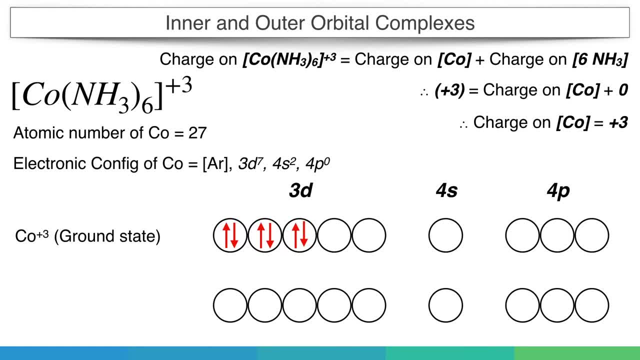 In this case, two d-orbitals, one s-orbital and three P-orbitals are shifted in total, So these are all empty ions. We can see that this is the cobalt p orbitals are involved in hybridization, So it is called as D2- sp3 hybridization. 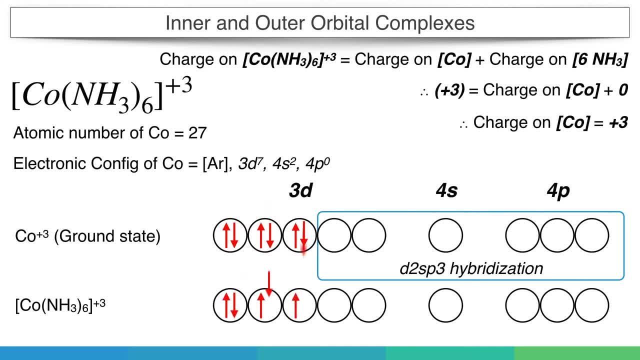 Please note here that the s and p orbitals involved in hybridization are of valence shell, that means 4th level, while d orbital is from the level below the valence shell, that is, 3rd level or inner orbital. This type of complexes where inner d orbitals are involved in hybridization. 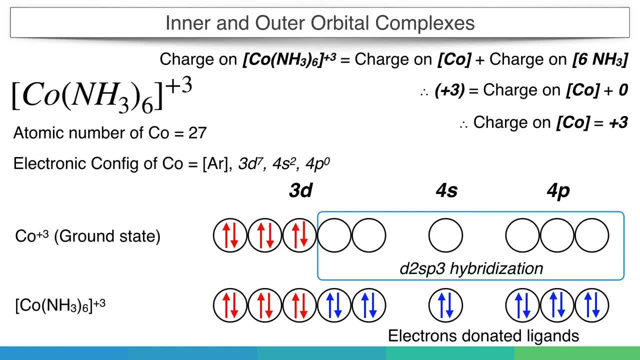 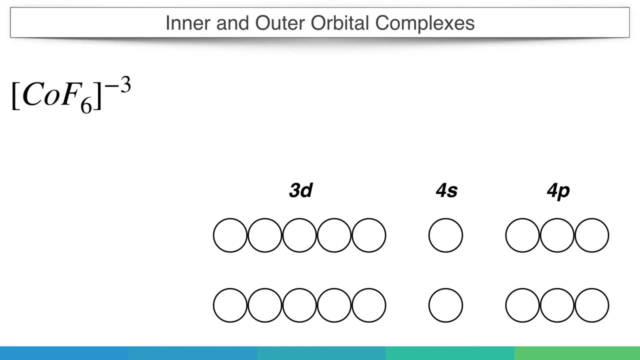 are called as inner orbital complexes. Also, as in the complex, all the electrons are paired. it must be diamagnetic, as observed in experimental results. On the other hand, if we try to explain the bonding in second complex, that is, hexafluorocobalt III, 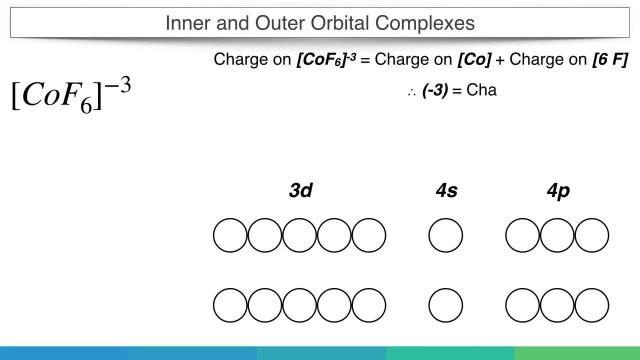 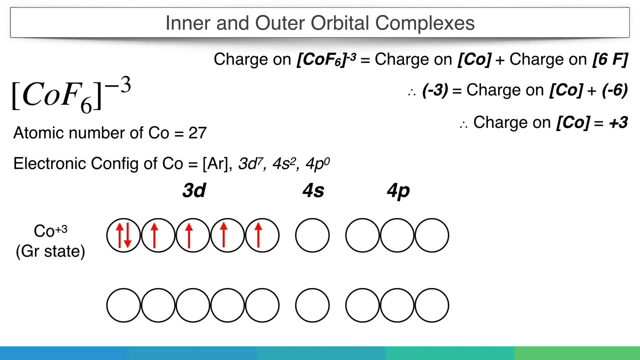 Again, the cobalt is in plus three oxidation state. So the same electronic configuration and the electrons can be arranged in 3d orbitals, leaving 4s and 4p orbitals empty. But in this case, as fluorine is weak field ligand, shifting of electrons does not take. 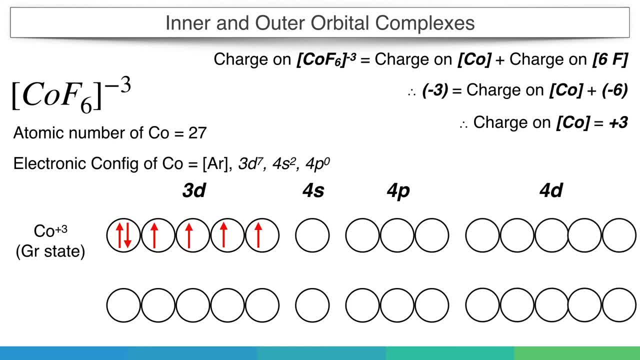 place. Instead, the outer d orbitals are involved in hybridization, So in this case, 1s orbital and 3p orbitals from valence shell, that is, 4th level, is involved. Also 2d orbitals of same level, that is, 4th level, are involved. This means outer d orbitals. 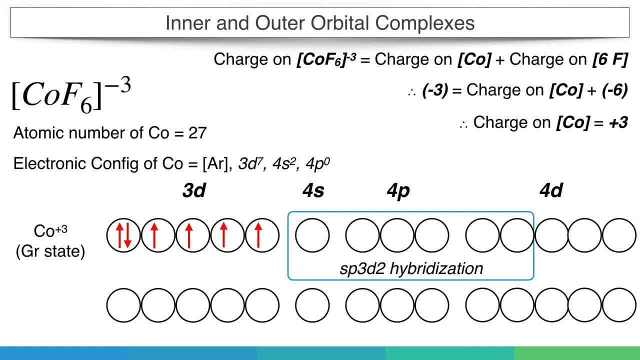 are now involved. We can write as it is: sp3- d2 hybridization, And now there are 6 empty orbitals available to accommodate 12 electrons coming from the ligands. You can see that here, as electrons are not shifted, they remain as unpaired electrons. 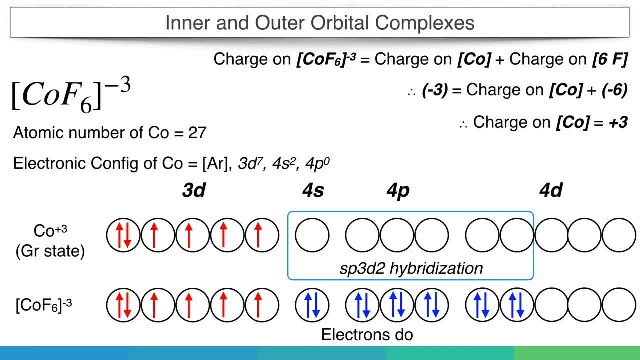 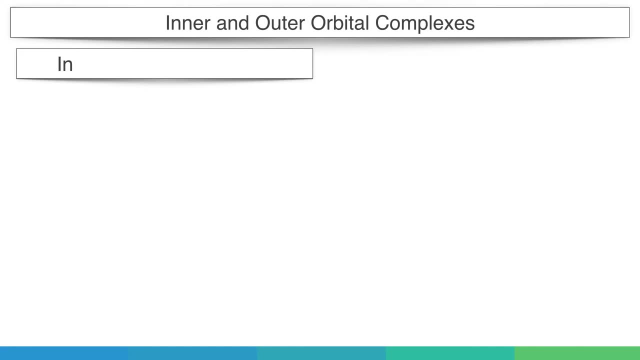 Thus this complex becomes highly paramagnetic in nature. So depending upon whether inner or outer d orbitals are involved in bonding, their magnetic properties gets changed. So let's try to distinguish between inner and outer orbital complexes. The complexes in which n-1d, ns and p orbitals take part in hybridization are called inner orbital. 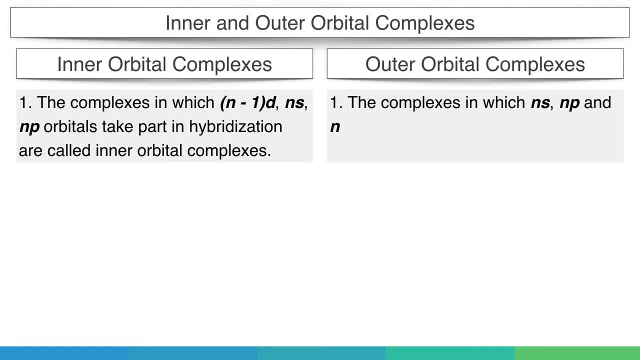 complexes. The complexes in which ns, np and nd orbitals take part in hybridization are called outer orbital complexes. Second: d2- sp3- hybridization takes place. sp3- d2- hybridization takes place. Third: electrons usually pair up. Electrons don't pair up. They don't match, They don't match, They don't.